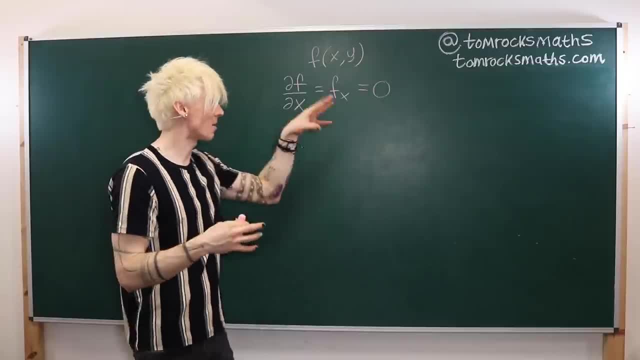 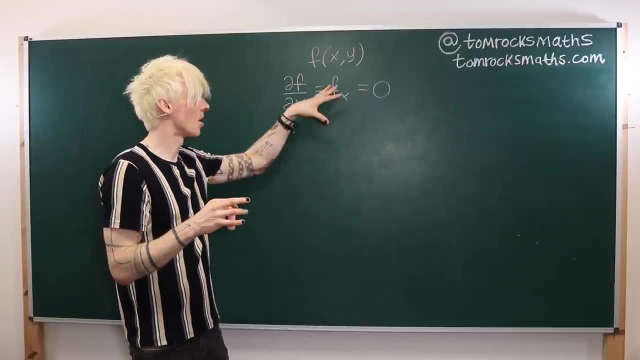 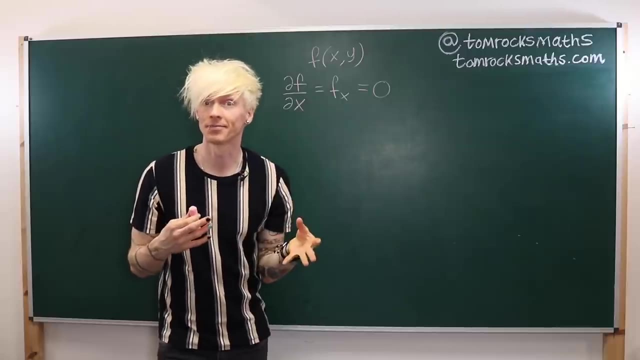 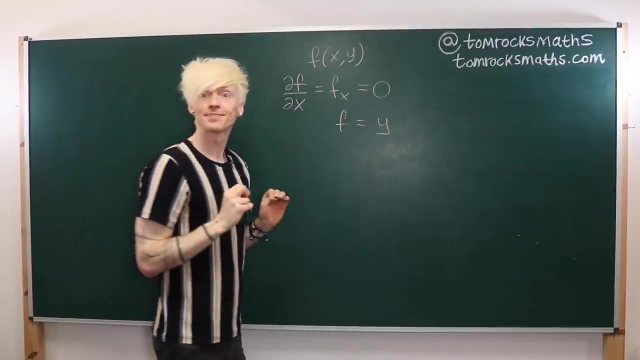 differentiate a constant, we get zero, and that would tell us how to integrate back up to get the solution. So here we want to think about what can I differentiate with respect to x so that I will get zero? One simple example might be if f was equal to y, If I take the x partial derivative of 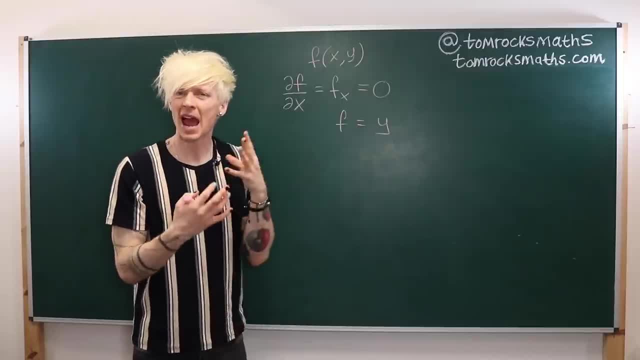 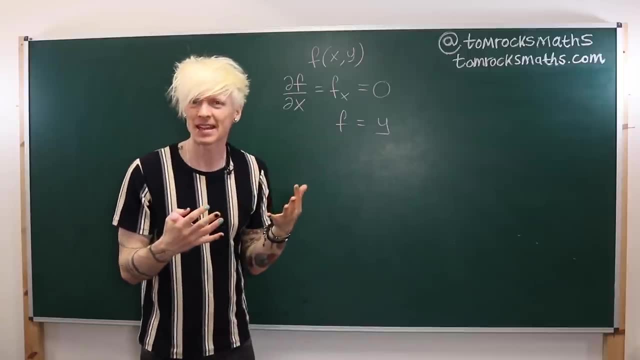 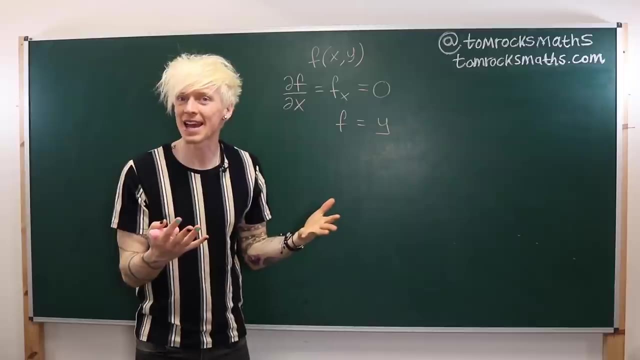 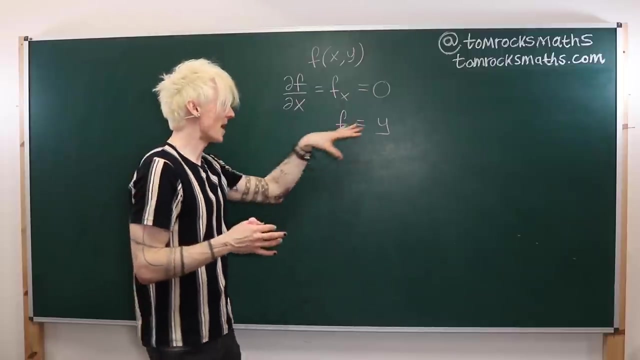 this function, then that is looking at how f changes in the x direction. But since f doesn't depend on x, it doesn't change in the x direction, and so therefore df by dx, partial, is indeed zero for this particular function. But there was nothing special about me picking y. What if I'd had? 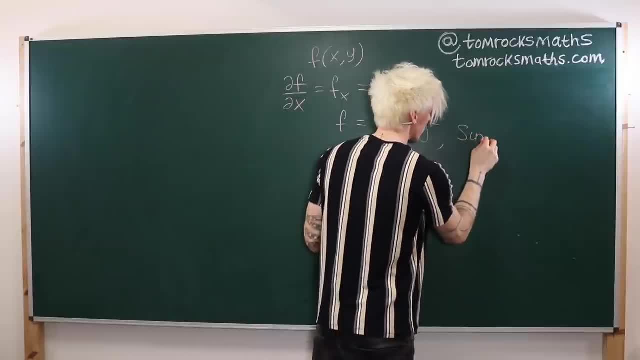 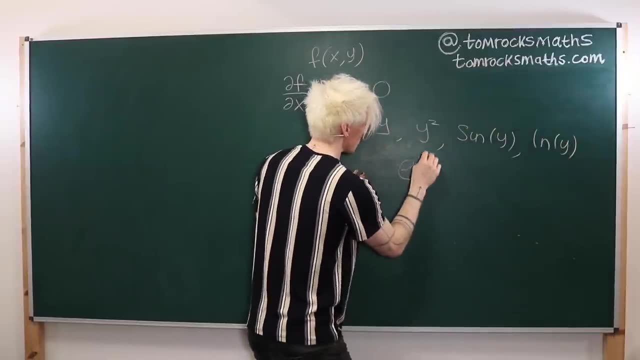 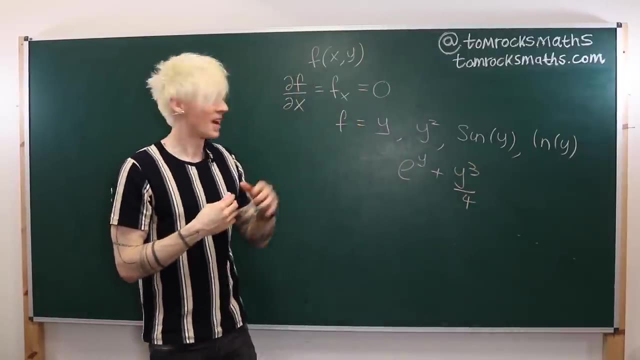 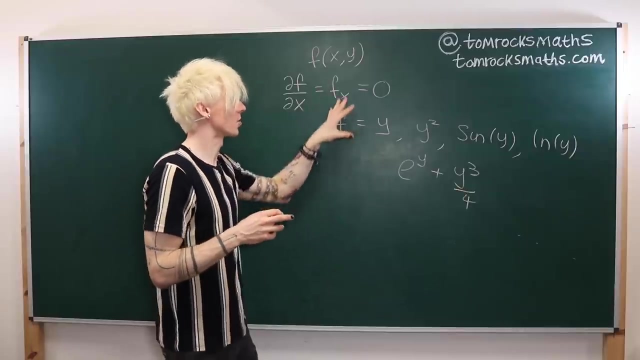 squared or maybe even sine of y, or log of y, or even e to the y plus y, cubed over 4, for example. All of these functions, when you take the x partial derivative, will give you zero. So they are all valid solutions to this PDE. 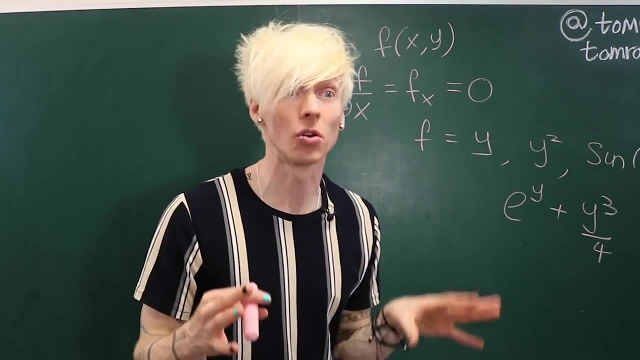 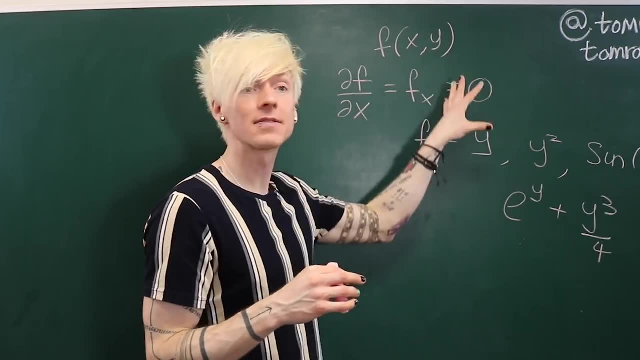 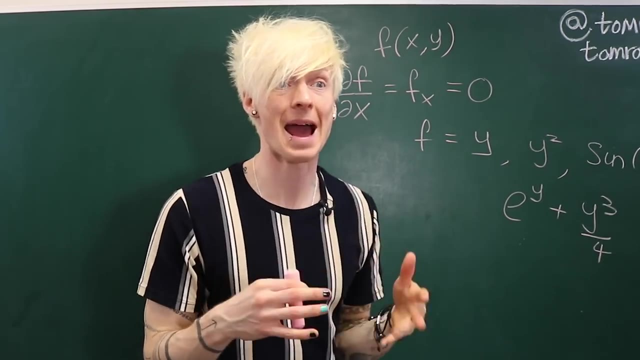 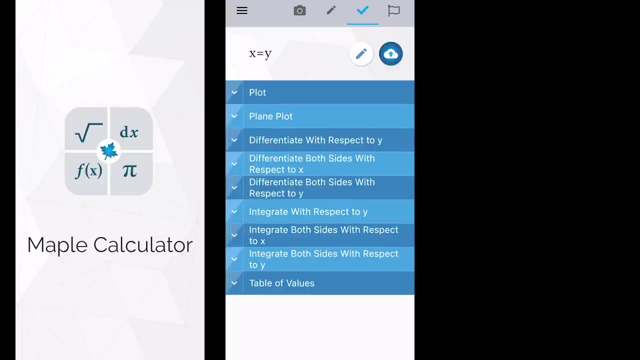 So, in fact, any function at all of the variable y will differentiate with respect to x to give us zero. And if you don't believe me, you can try this for yourself in the Maple Calculator app, Write any expression that's a function of y only, and when you click on the x derivative, 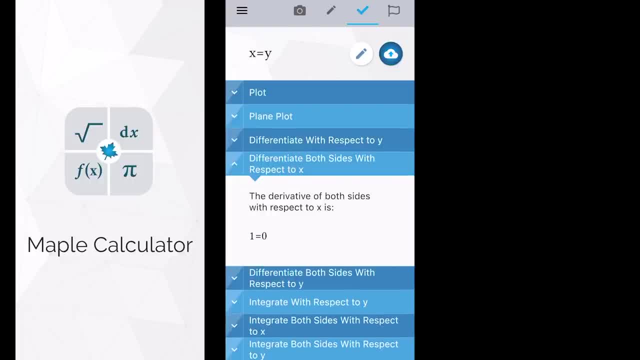 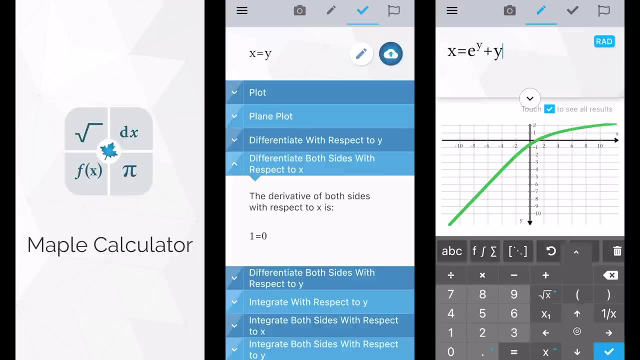 which is one of your options, you'll see that the answer is always zero, No matter how complicated the expression that you input. You can also, of course, see the y derivative for any weird and wonderful function that you can input, and I can assure you it is quite good fun. 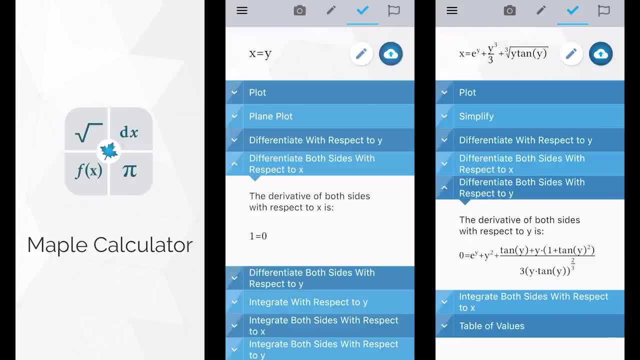 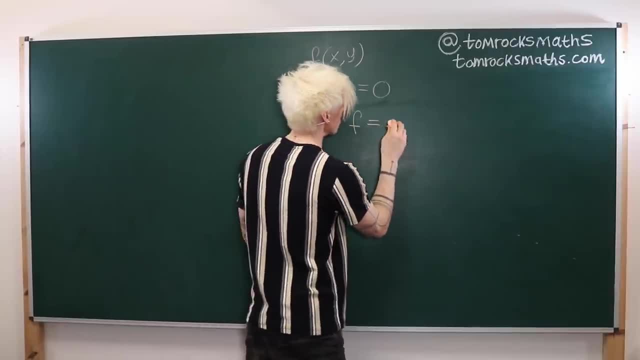 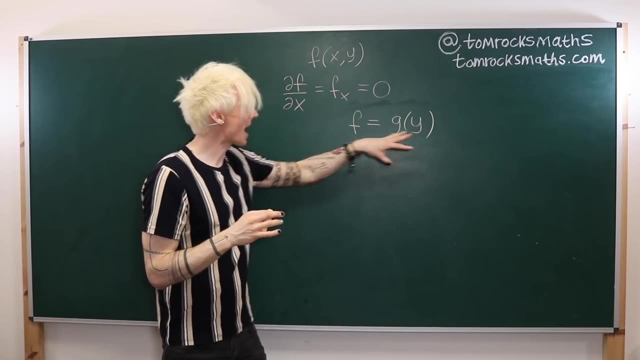 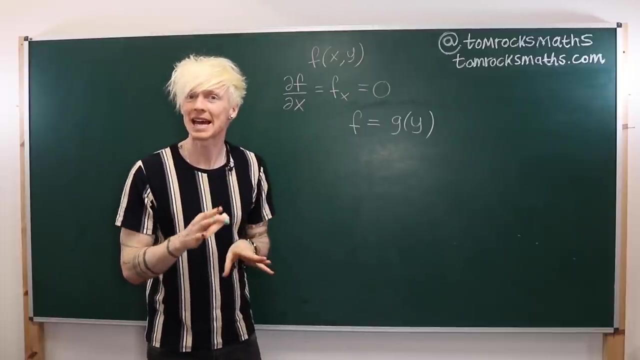 seeing just how messy and creative you can get with your function. So what this means for our PDE is that the solution f is equal to any function g of the variable y, Because when we take the x derivative of a function of y only, as we've seen, we always get zero. 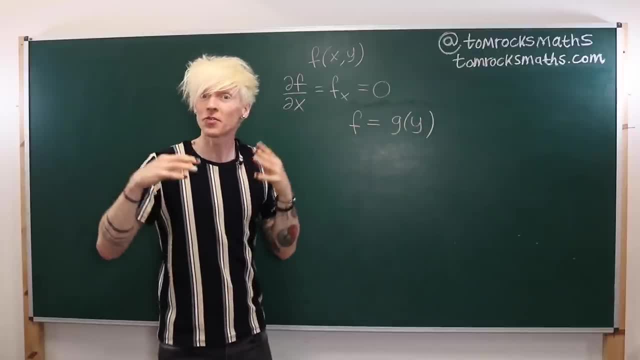 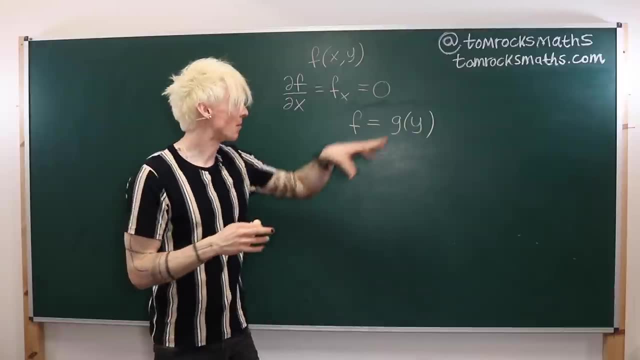 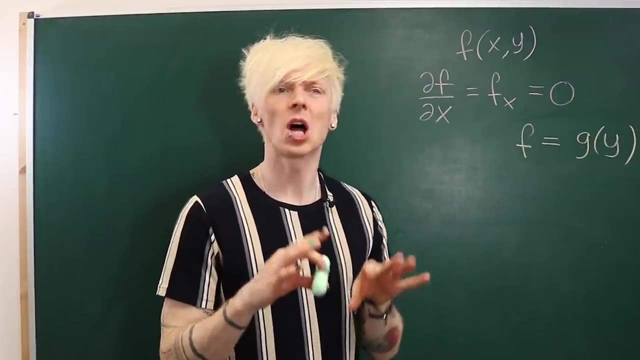 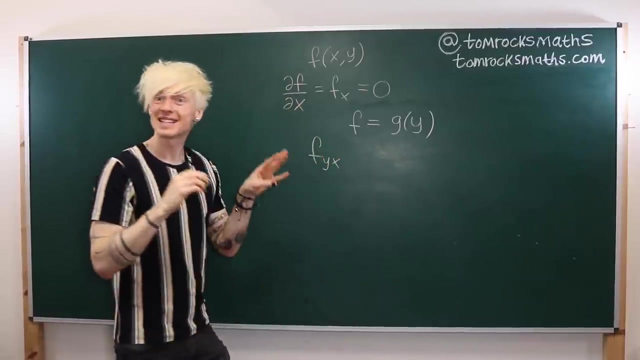 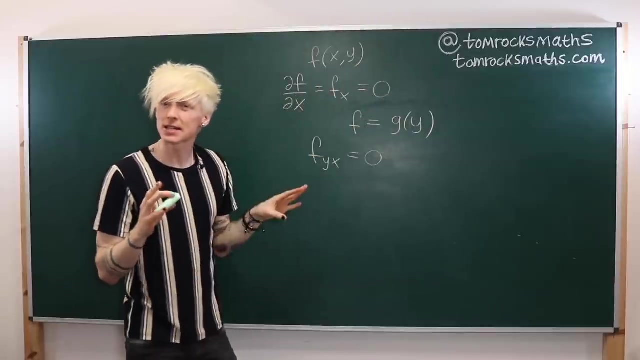 And here you can think of this integration function as playing the role of the integration constant plus c, and we're going to see this concept appearing in the next few examples. Now let's try something a little harder. so let's suppose we have two derivatives: d2f by dy, dx is equal to 0.. Now in our first example we 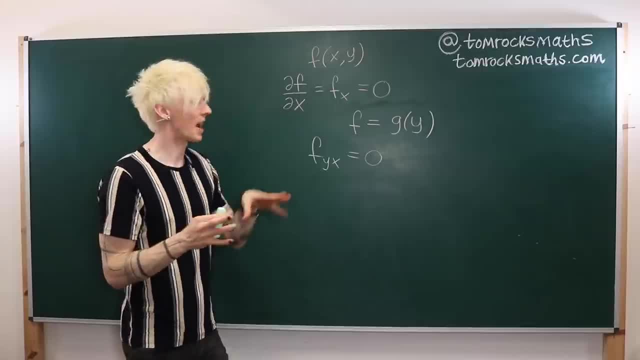 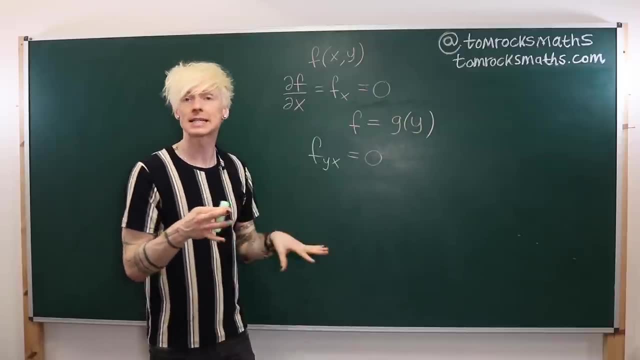 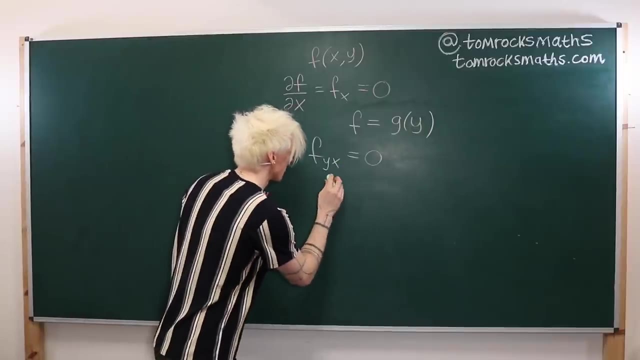 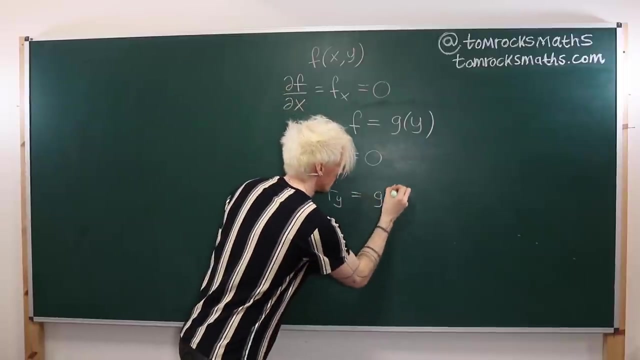 had a single partial derivative in x and we solve that by integrating with respect to x and thinking carefully about what would differentiate to give zero. So let's do the same here, So we can integrate with respect to x and say that df by dy is equal to a function g of y, Just as before, if I take the x. 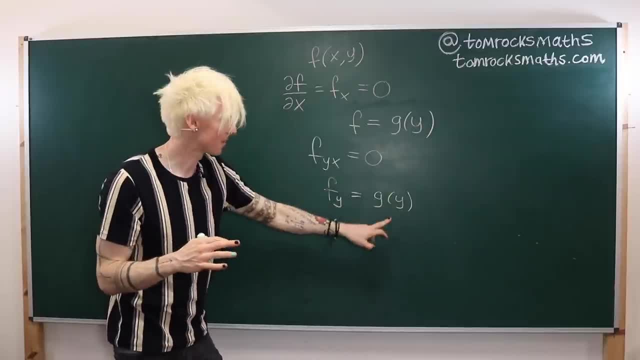 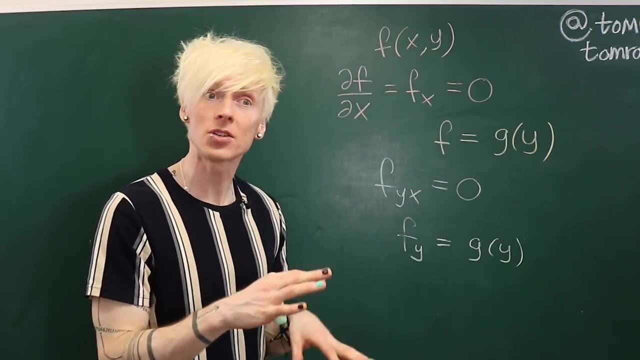 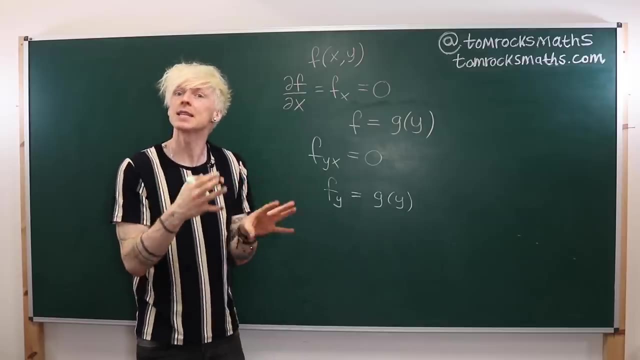 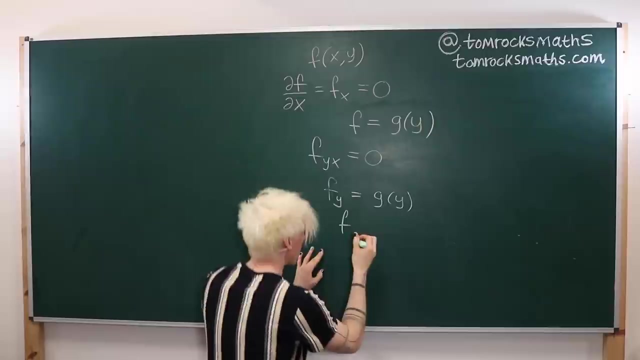 partial derivative of this function of y, I'll get 0. So it does indeed satisfy, f is 0.. Next, we need to integrate both sides with respect to y. So let's just go ahead and try that and see what happens. So if I integrate the left with respect to y, I get f and then the right. 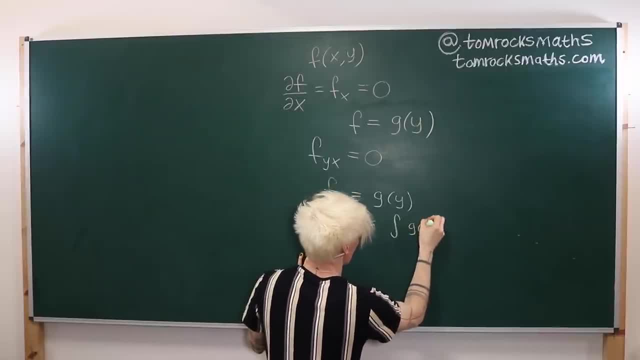 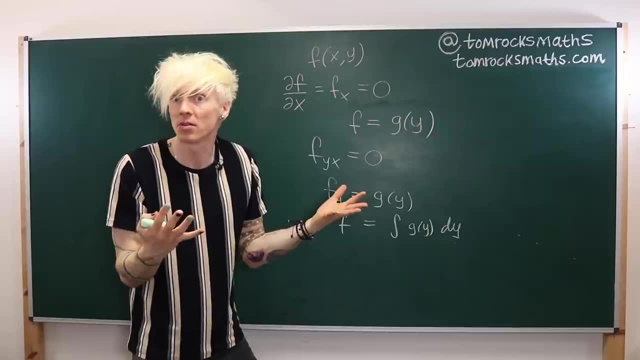 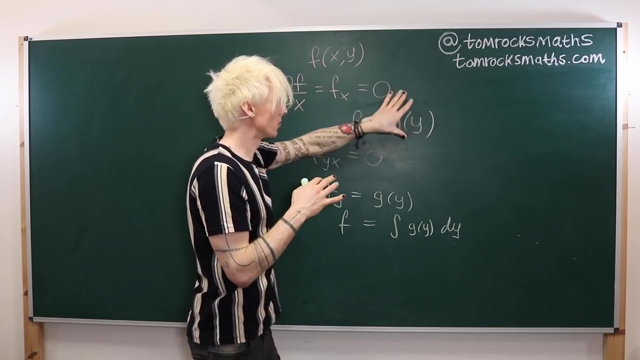 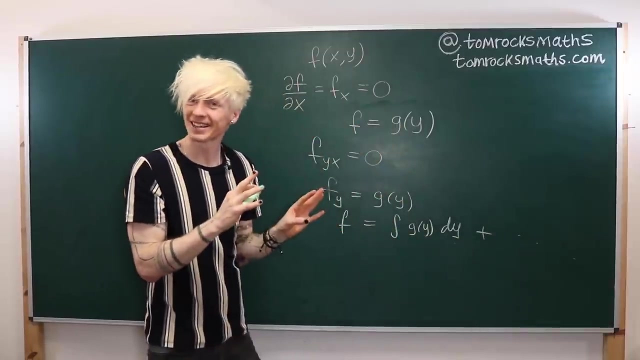 is going to be the integral of g of y, and we don't know what this function g of y is, so I can just write it as the integral of some unknown function. And then, similar to how, here we said, differentiation of function of y with respect to x gives me 0, my integration constant has: 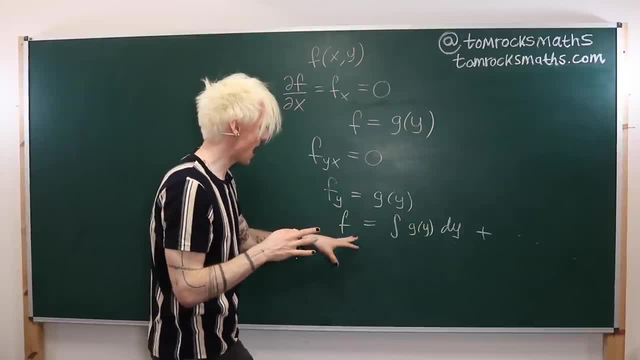 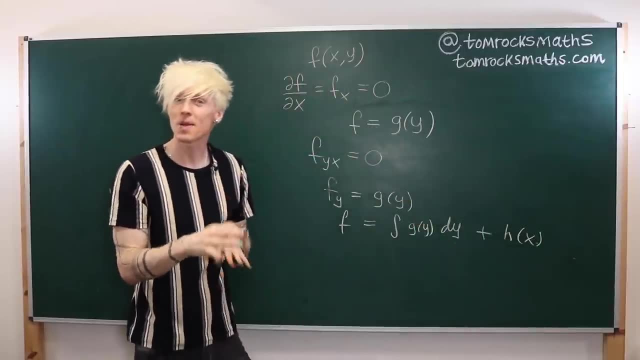 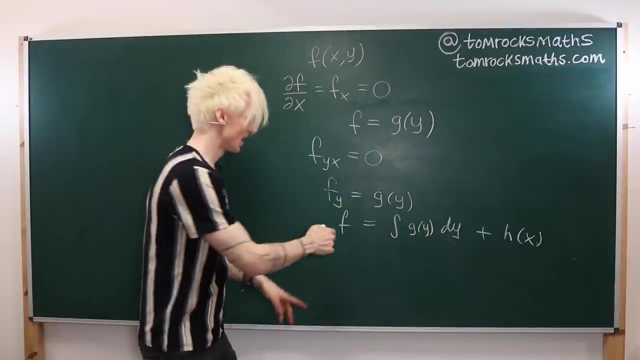 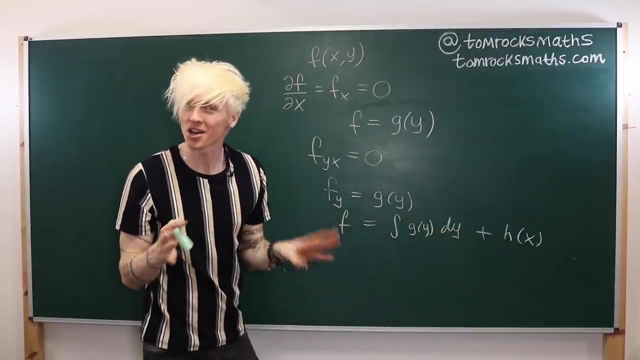 now become an integration function. so any function of x- so let's call it h- of x, when differentiated with respect to y, will disappear. So just to check this makes sense, this is my f. then differentiating this expression with respect to y as a partial derivative gets rid of the. 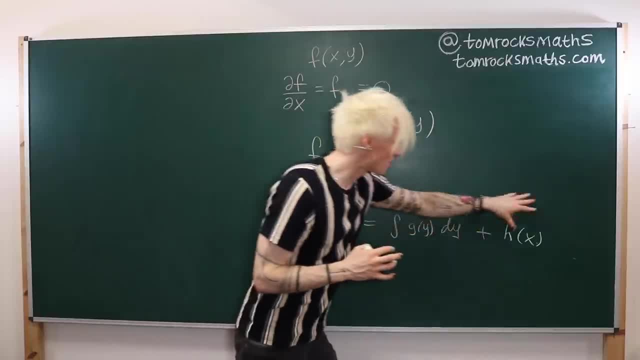 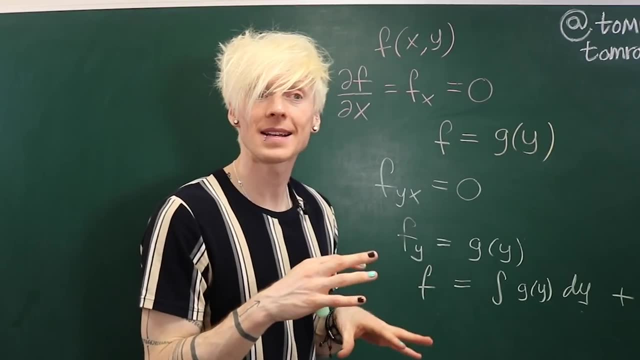 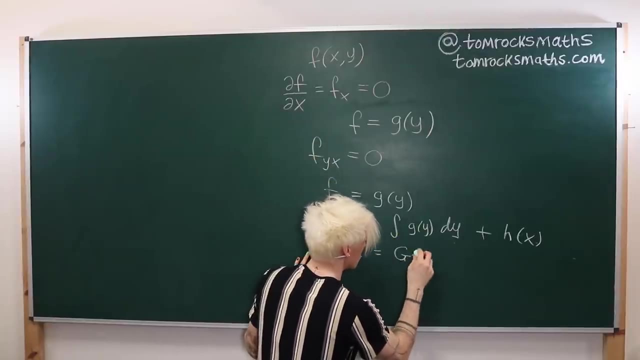 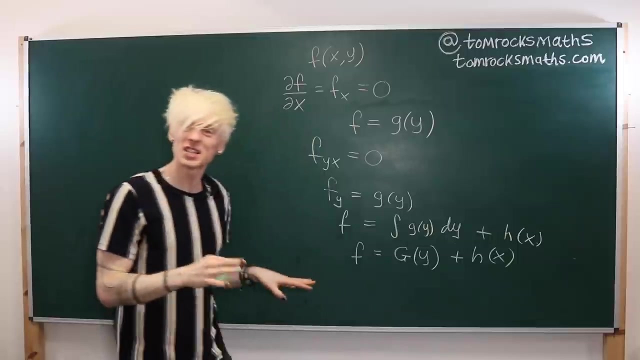 integral, so I get g, and then this general function h will completely vanish, because it's a function of x only. We can in fact simplify this even further, as we can say: the integral of a function of y just gives me another generic function of y. So we could specify that capital G of y is the 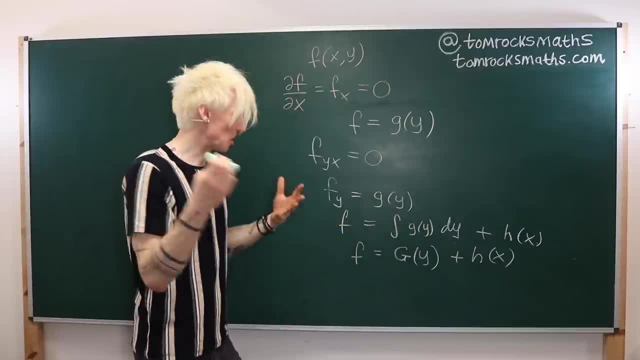 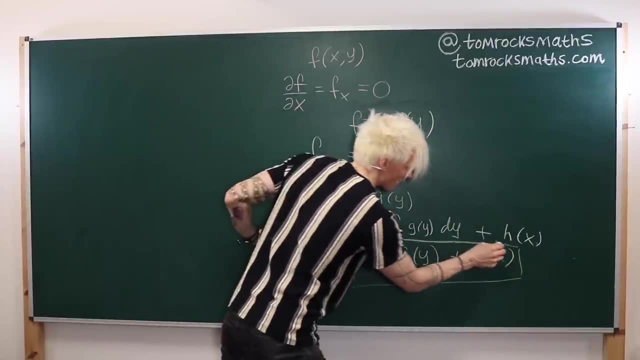 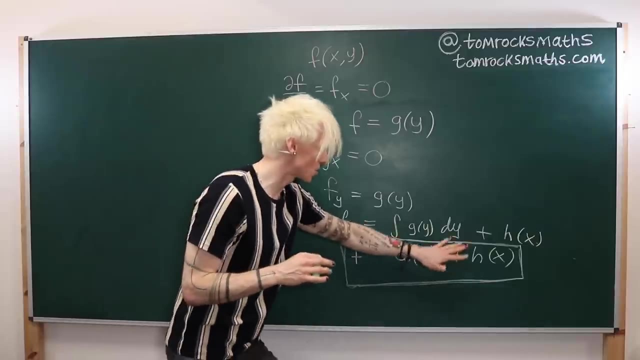 integral of lowercase g of y, but ultimately it doesn't really matter. The key concept here is that if I have any function f which has some function of y plus some function of x, then when I have any function f which has some function of y plus some function of x, then when I 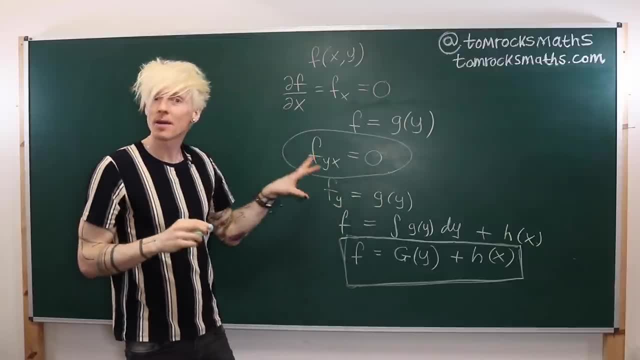 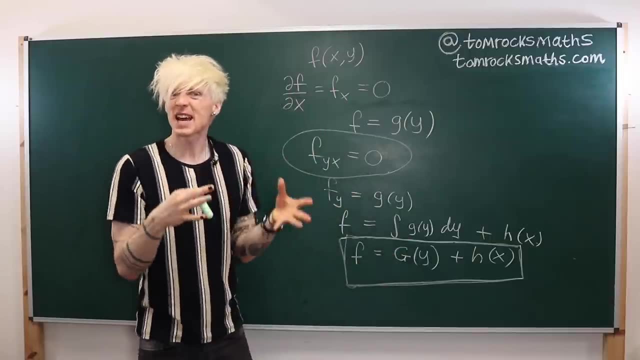 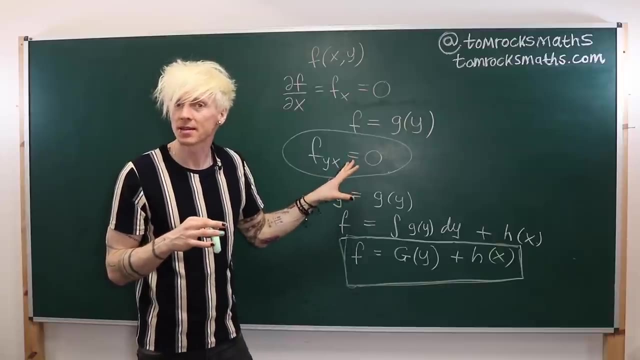 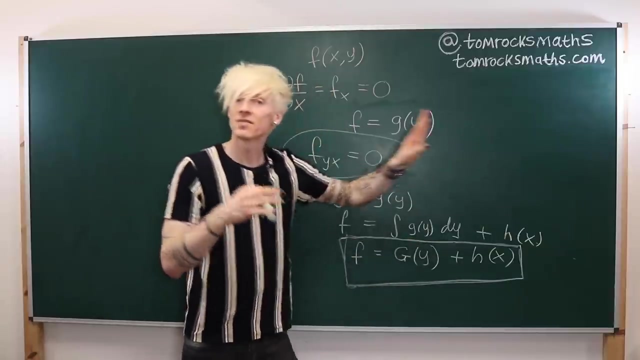 have any function f which has some function of x, then when I do an x and y partial derivative on this function I will get 0 and this makes sense. we can double check to see if this is indeed a solution to this PDE. So if this is my f, if I take my y derivative, the x function vanishes and I 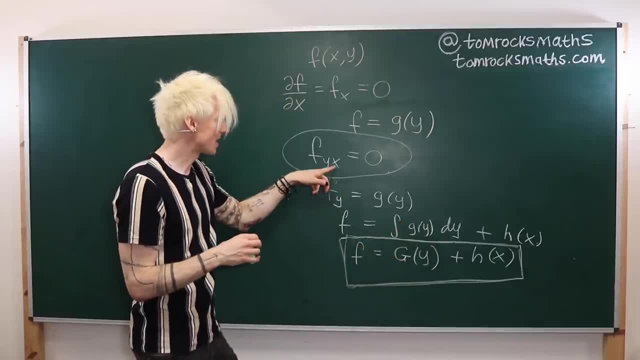 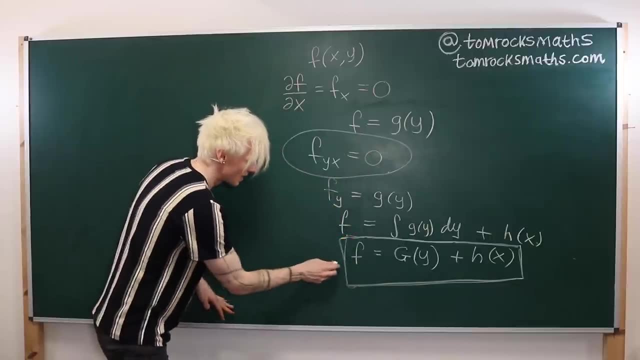 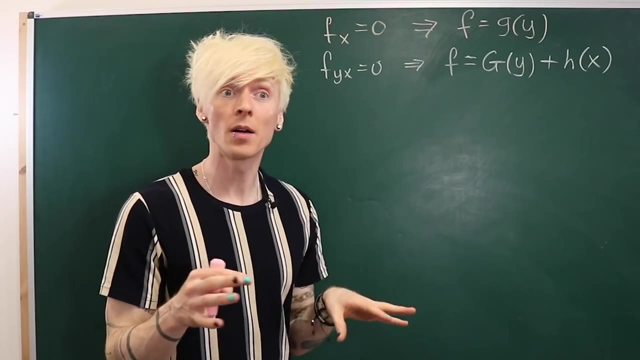 get something here involving y and then, when I take the x derivative, the y function vanishes, so I will get back to 0.. So this is indeed the most general form of solution to this second order PDE. So far we've only looked at 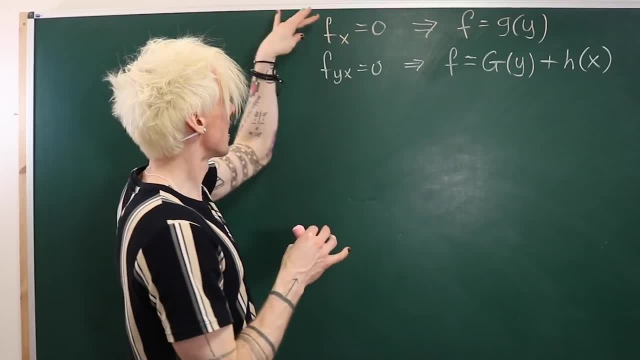 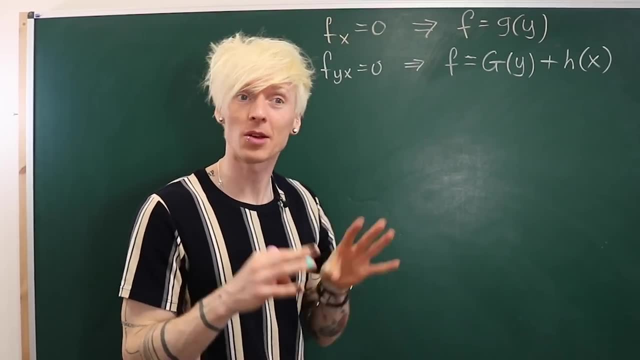 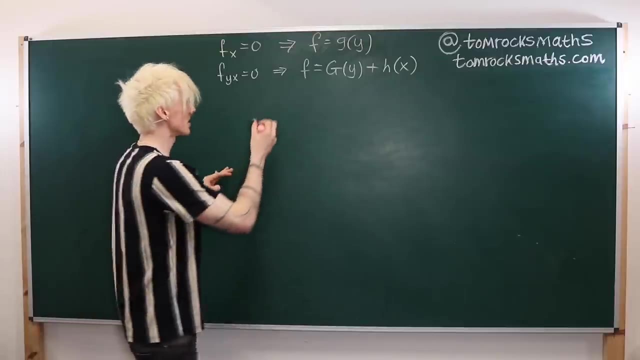 simple PDEs in the sense that in both cases we have them equal to 0. They were homogeneous, partial differential equations. Now let's look at something slightly more complicated. So we're going to consider a function u of x- y, so again a function of two. 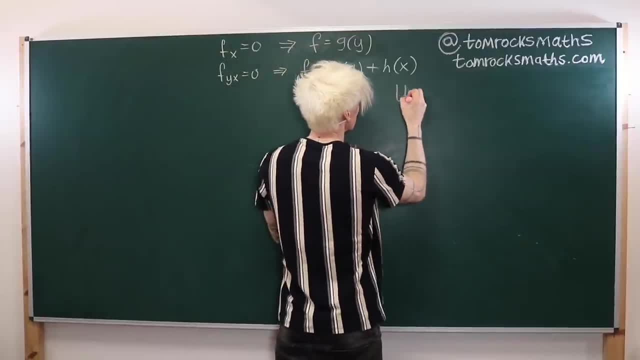 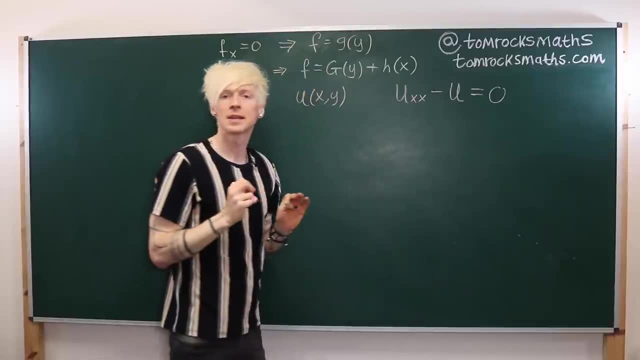 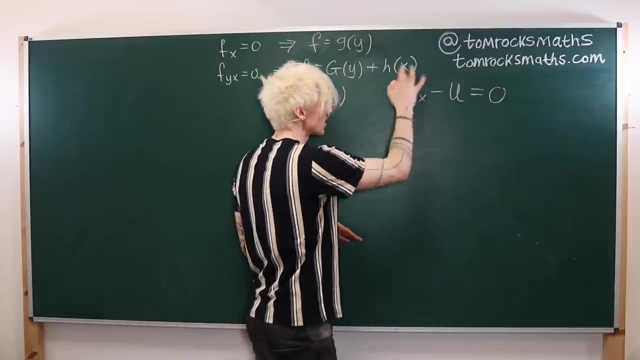 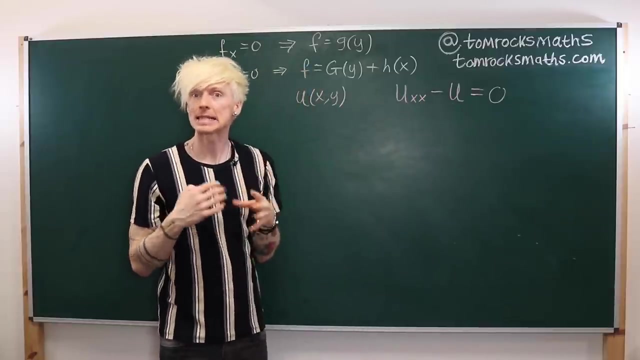 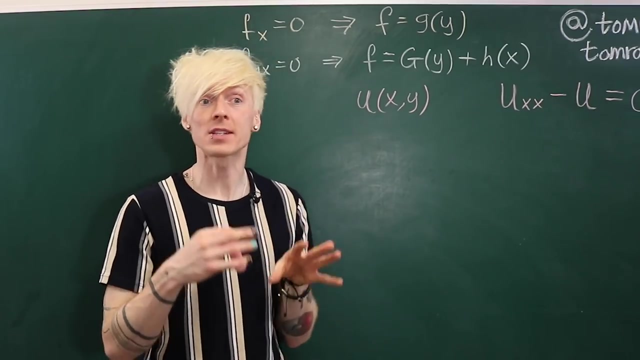 variables, and this is going to satisfy uxx minus u is equal to 0.. So now we have two terms involving our solution, u. we've got a second order, x derivative, and the actual solution or function u itself. Looking at this equation, we can see it's going to be a little trickier because our previous 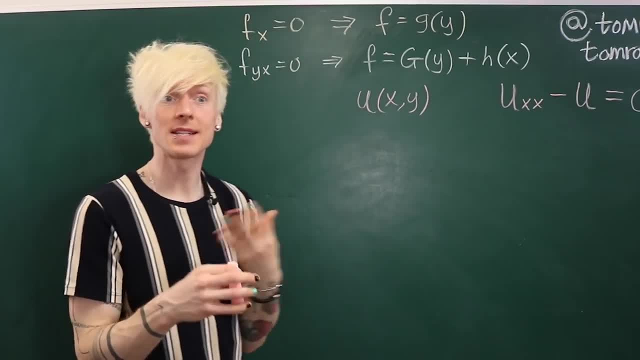 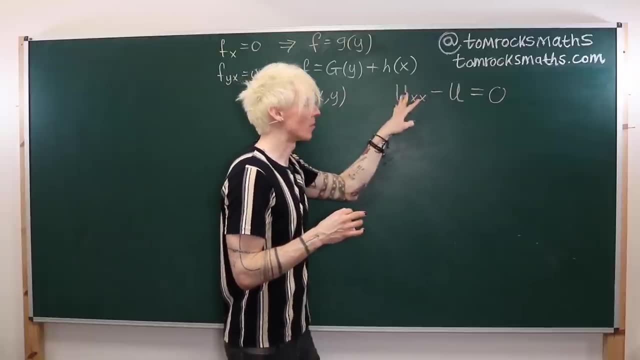 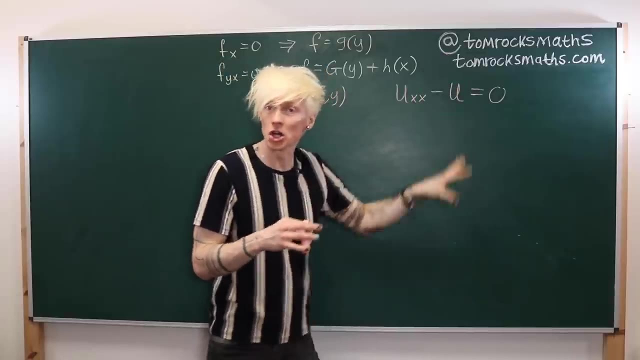 approach of just integrating both sides of the equation unfortunately isn't going to work, Because if I were to integrate with respect to x, this term would be fine, but then I'd be left with the integral of the unknown function that we're trying to solve for. So we're going to have to take a slightly. 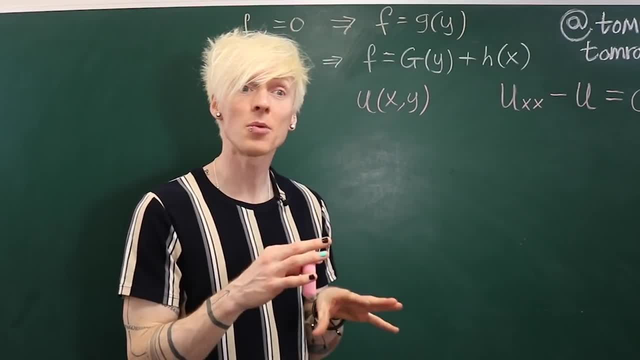 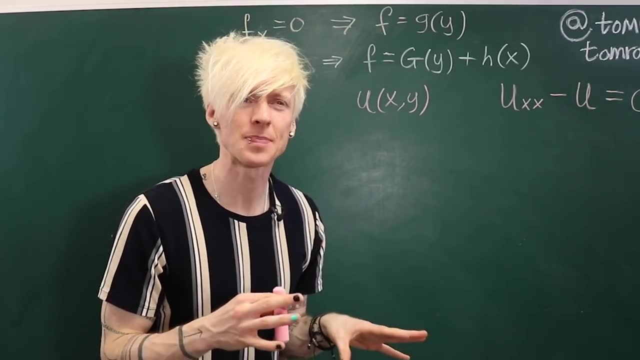 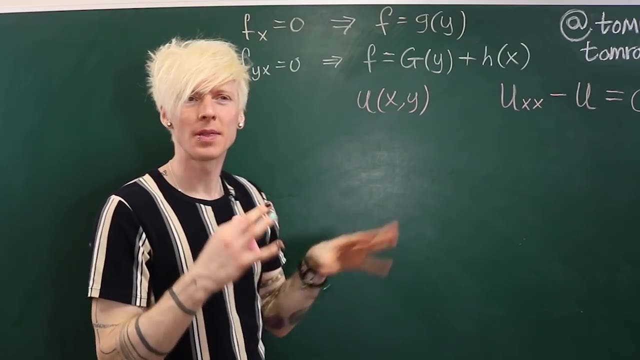 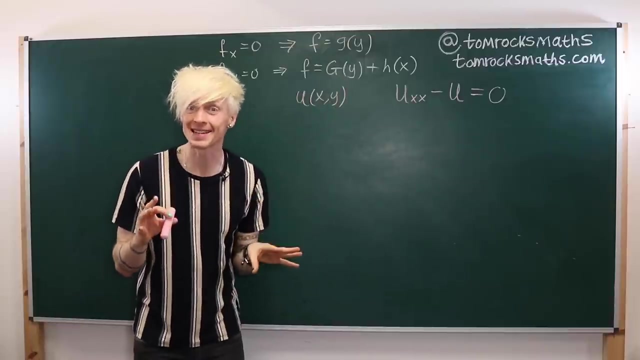 different approach. If we think back to how we dealt with our first equation, we used our knowledge of ordinary differential equations to help us to come up with a sensible way of trying to solve the PDE. So let's try something similar for this one. Let's first pretend- and I do mean pretend- that 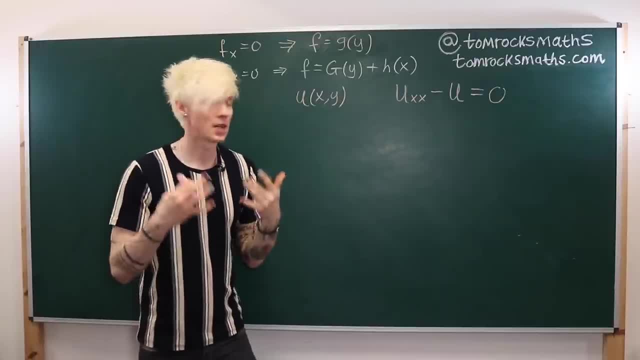 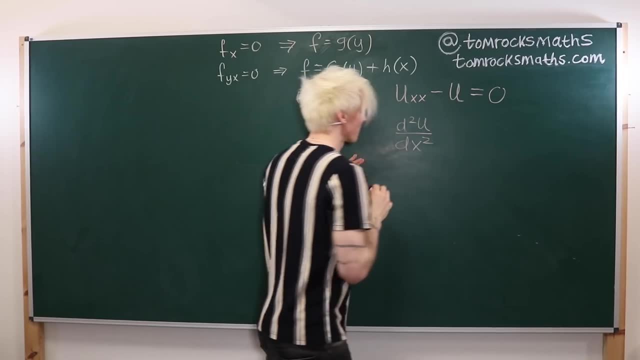 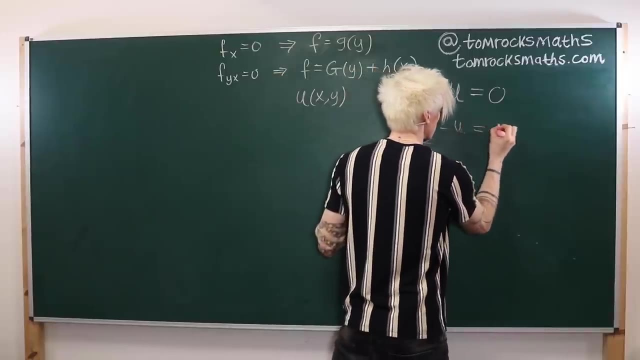 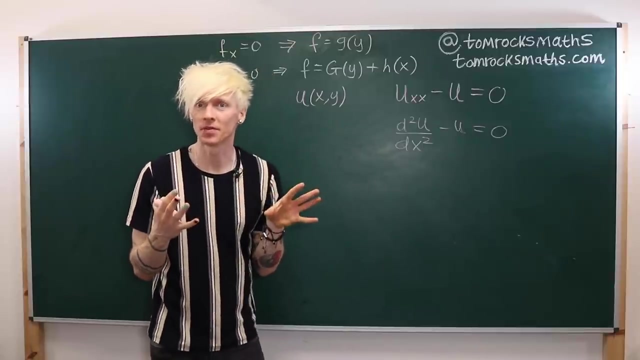 this is in fact an ODE. So let's suppose that we were solving d2u by dx squared, where these are now full derivatives in x minus u is equal to 0.. So let's just run with this And see if we can get anywhere useful, Because it certainly helped us here with 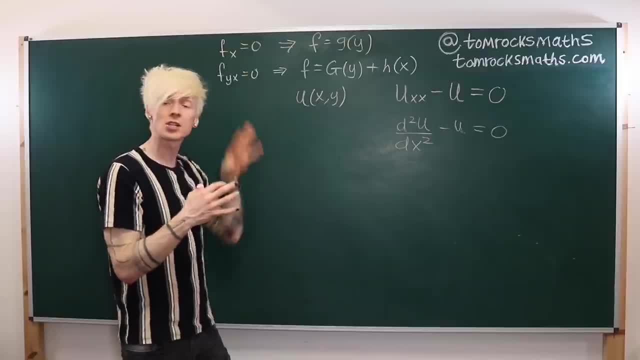 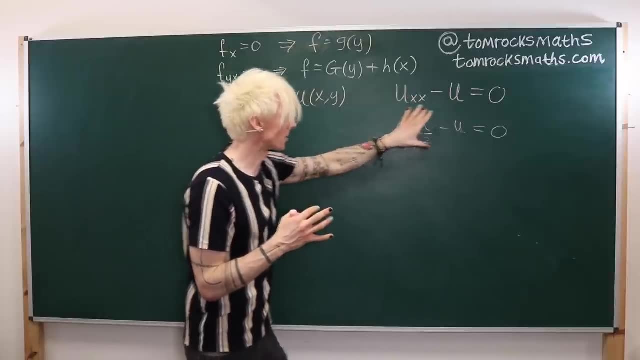 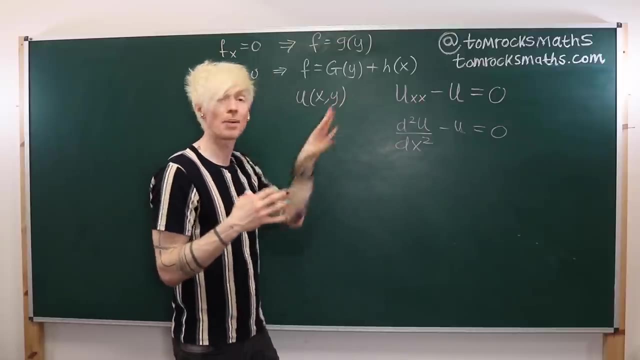 thinking about the fact that the solution was a constant, precisely because it differentiated to give us 0. So maybe we can get something by looking at the solution of the ODE and then trying to relate it back to what might happen in the partial derivative case. To solve this equation we would try a solution of 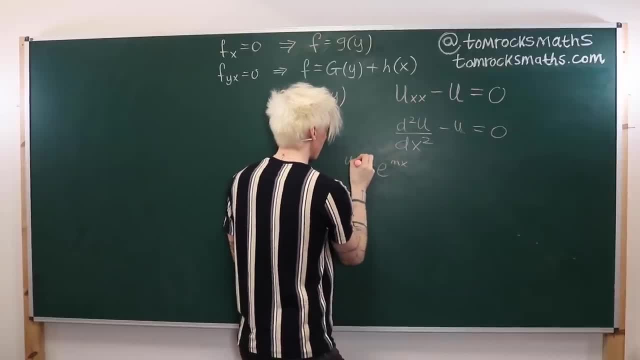 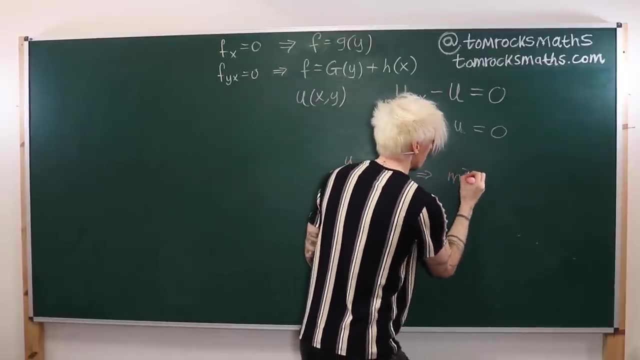 the form e to the n. So let's say that we've got a solution of the form e to the n plus e to the minus x. So we can just plug that in to get our auxiliary equation, which here will just be m squared. 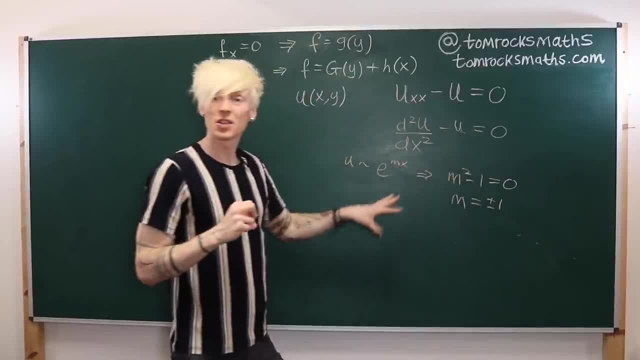 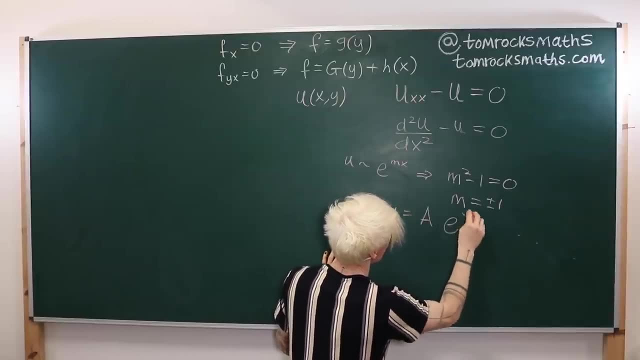 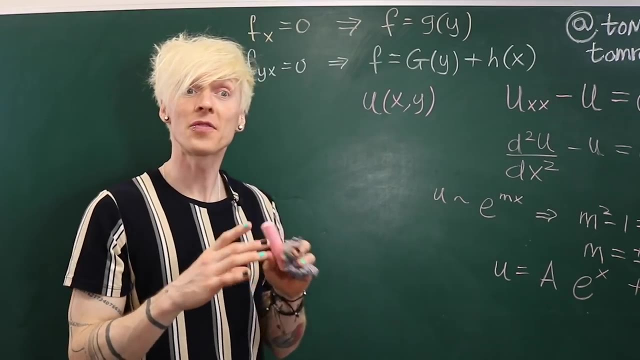 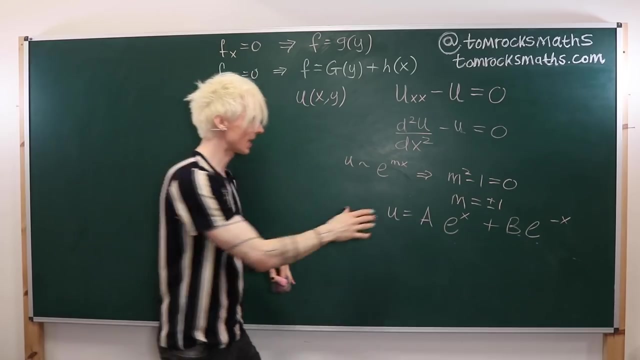 minus 1 equals 0, which tells us that m is plus or minus 1.. And so for this ODE our solution is: u equals a, e to the x, plus b, e to the minus x. Now, in our first two examples we've seen here that integration constants, which here: 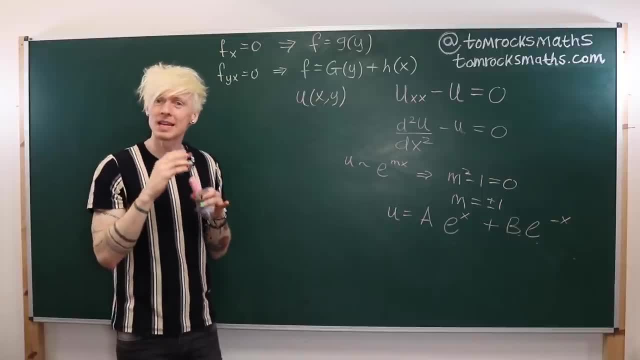 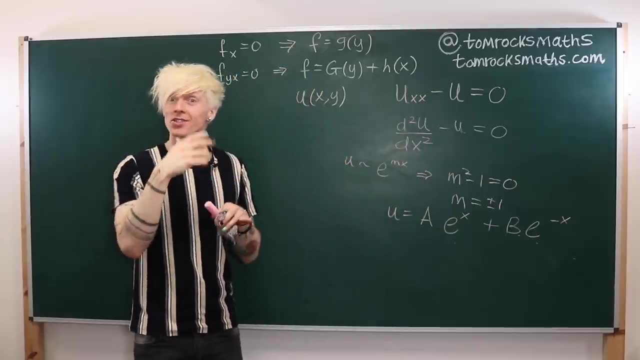 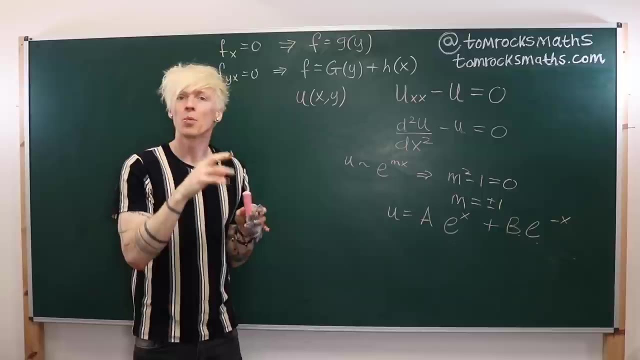 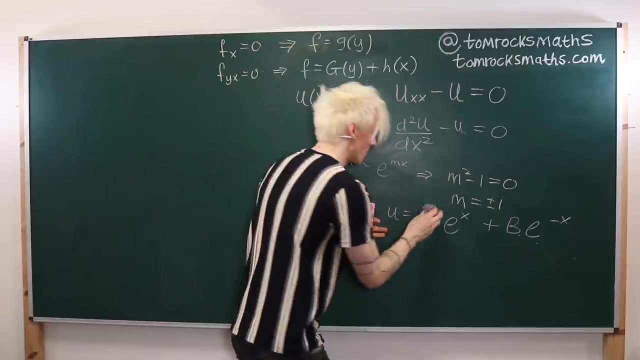 are a and b are replaced by integration functions, And here we have two x partial derivatives. So that means our integration constant, or integration function, will be dependent on y only. So, So, So why don't we try replacing a, which is our integration constant, by, let's call it, 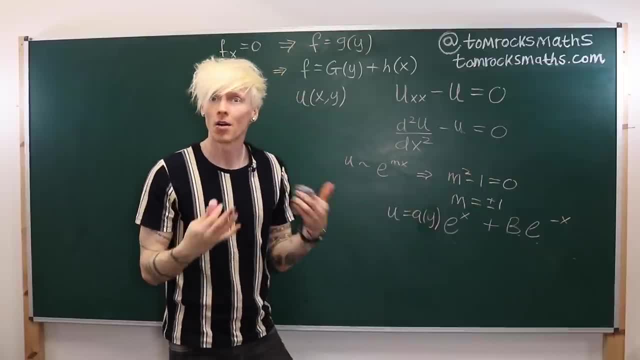 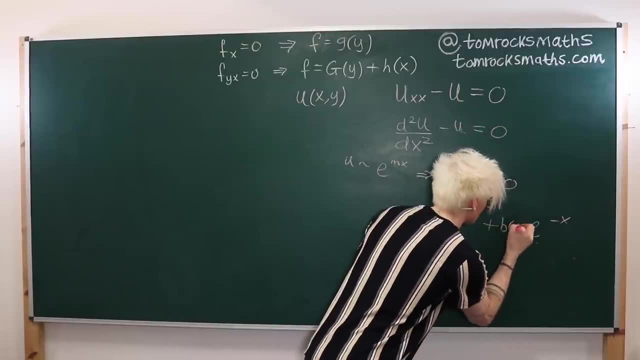 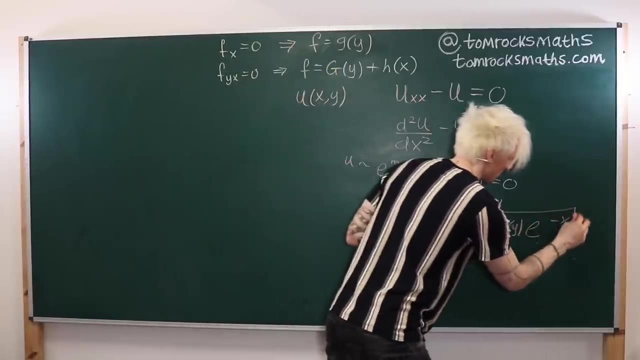 lowercase a of y, So a function of y. And similarly, let's replace b, which was just a constant, by lowercase b, which is now a function of y. So this is, I would argue, a plausible solution. So 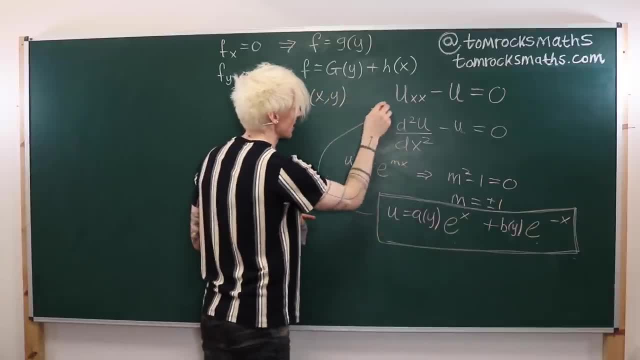 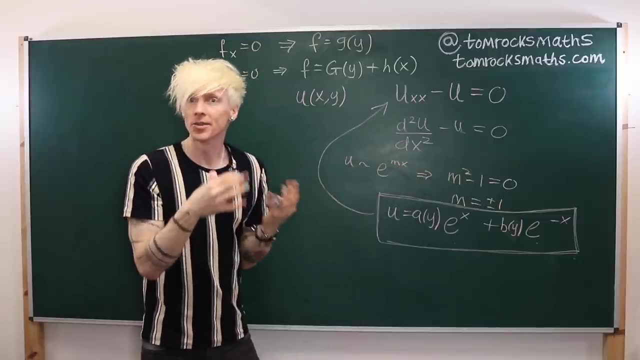 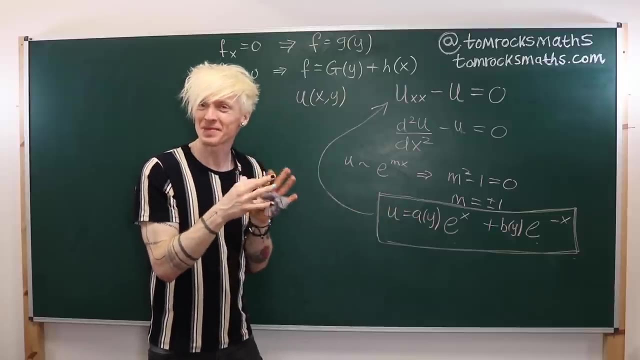 So, So So that's the solution to our PDE, And this came from pretending that this was an ODE, solving the ODE using our known methods, which here was the auxiliary equation, And then, as I mentioned at the beginning, cleverly turning the problem back into something that 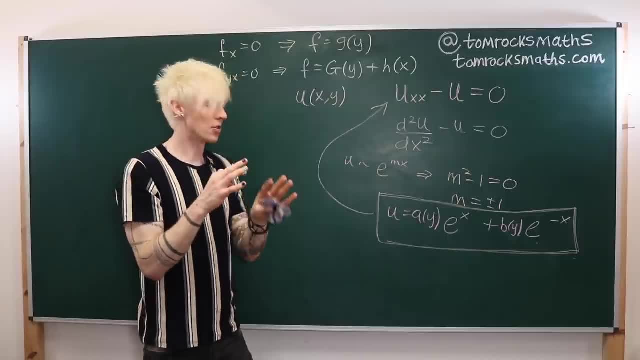 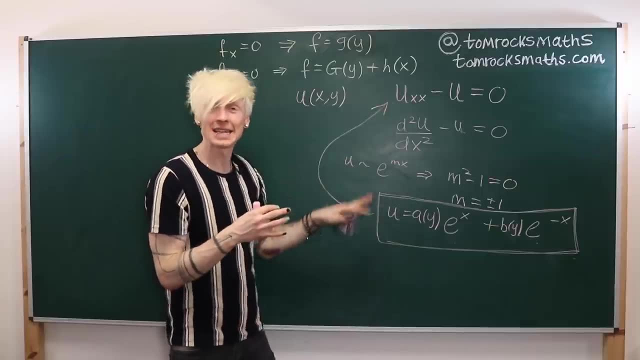 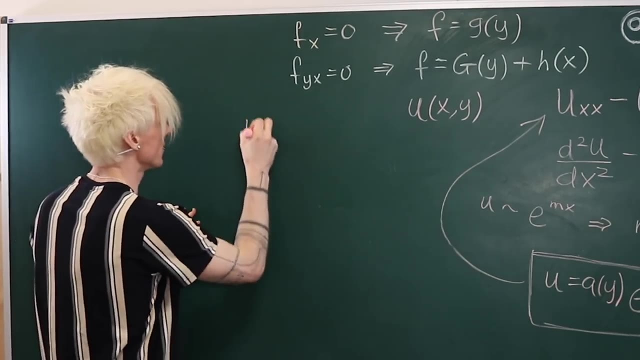 relates to partial derivatives. Now, of course we don't know this is the solution yet. We're I've just said this is a sensible thing to try, so let's plug it in and see if this will indeed satisfy our PDE. Taking the first x derivative du by dx. so 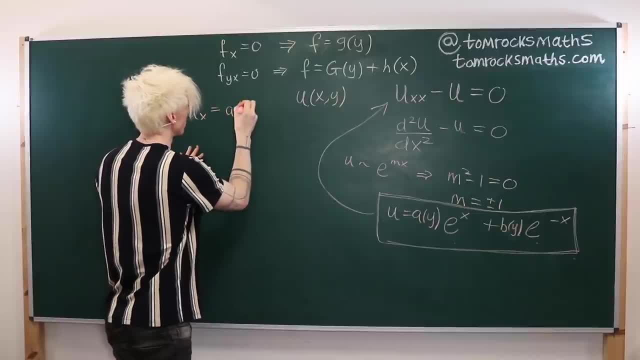 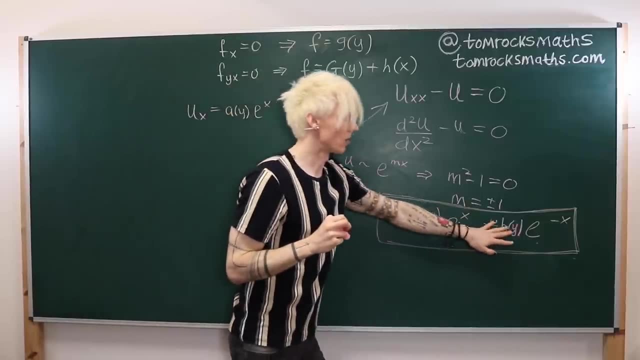 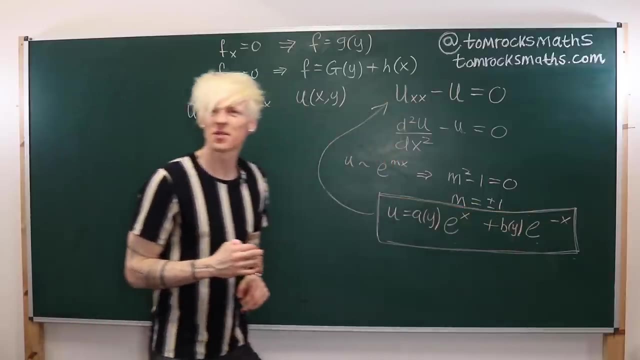 this is a function of y, so it's unchanged. then I differentiate e to the x, which just gives me e to the x. then I've got a function of y again, so that's unchanged by the x partial. but I'll get a minus from the exponential, so I'll get 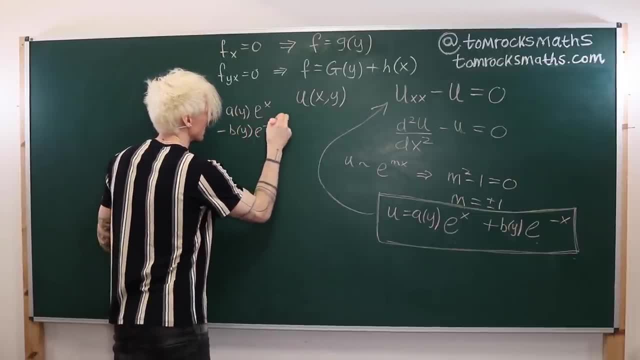 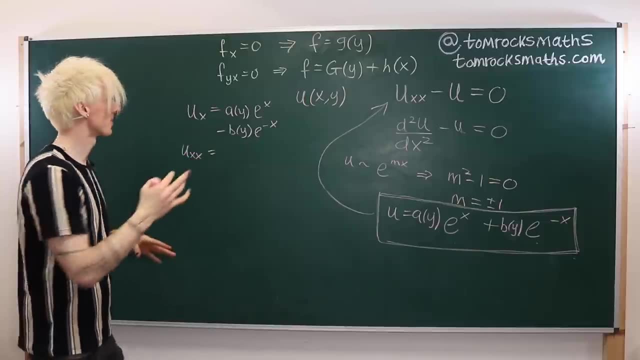 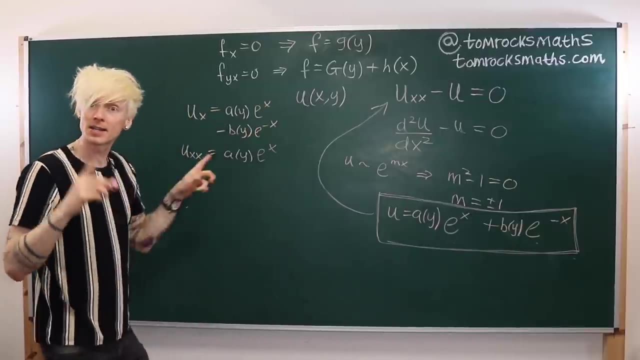 a minus by e to the minus x. and then my second derivative is to differentiate this with respect to x. so again the a isn't touched and I'll just get another e to the x, and then I'll get a minus coming down again. give me plus b to the.